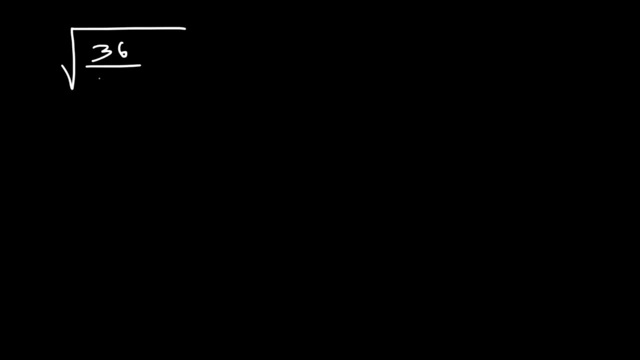 What is the square root of 36 divided by 49?? And also negative root 121 over 169.. Go ahead and try these two. The square root of 36 is 6, and the square root of 49 is 7.. 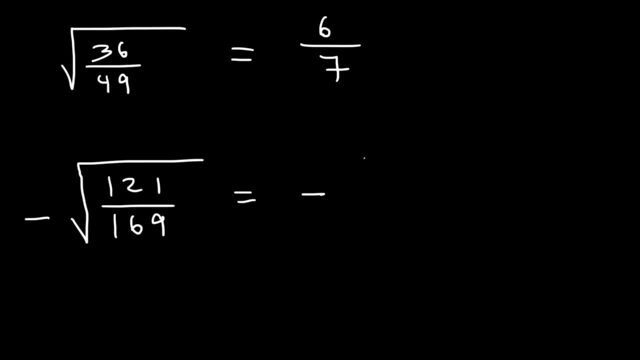 That's all you need to do. for this one, The square root of 121 is 11, and the square root of 169 is 13.. And what about this one? Negative 81 over 144.. Go ahead and simplify that example. 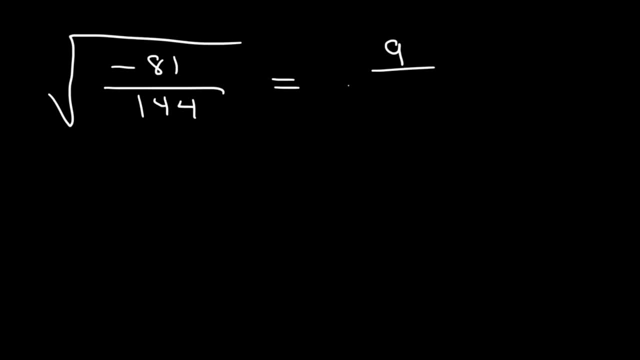 The square root of 81 is 9,, the square root of 144 is 12.. And because we have a negative sign on the inside, we need to include the imaginary number. So let's do this: The square root of 61,. negative root of 149, and the square root of 149 is 13.. 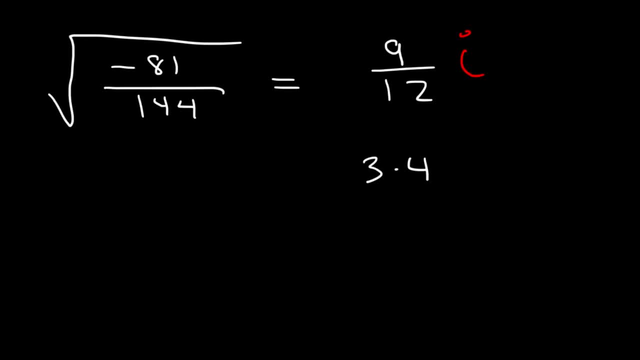 Now we can reduce 9 over 12.. 9 is basically 3 times 4.. I mean not 3 times 4, it's 3 times 3.. 12 is 3 times 4.. So we can cancel a 3.. 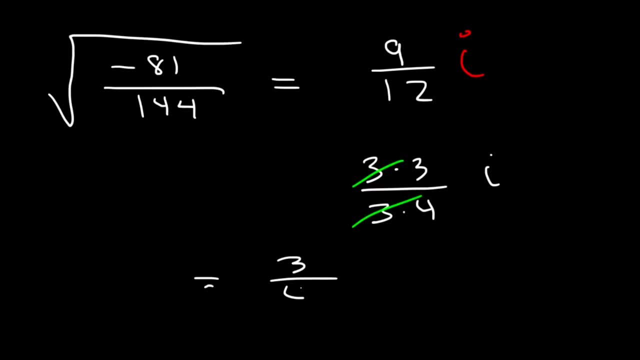 So therefore, the answer is 3 over 4 times i. Now what is the square root of .16?? what do you think the answer is? notice that there's two digits to the right of the decimal point and when you take the square root, the answer should only: 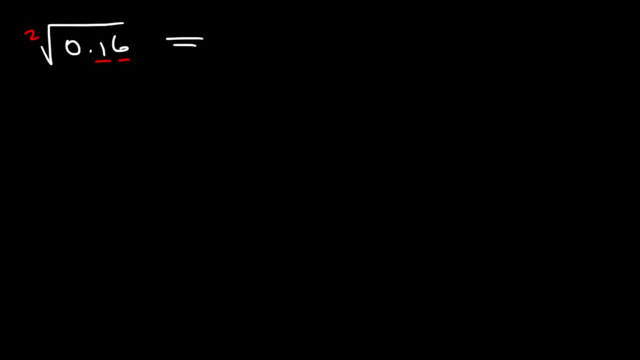 contain one digit to the right of the decimal point. the square root of 16 is 4, so it's going to be point 4, since it has one digit to the right. what about the square root of .0025? notice that there's four digits to the right of the 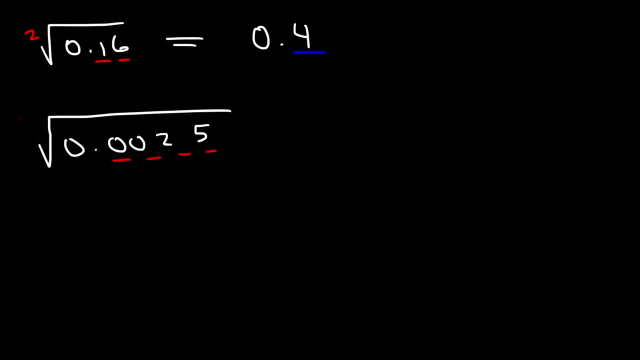 decimal, and 4 divided by 2 is 2, so the final answer should have two digits to the right of the decimal point. the square root of 25 is 5, so this is going to be .05. as you can see, it has two digits to the. 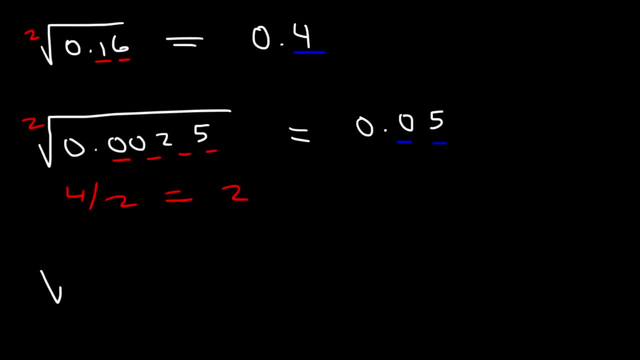 right of the decimal point. and now, what about this one, the square root of .00081. notice that we have six digits to the right of the decimal point. 6 divided by 2 is 3, so the final answer should have three digits to the right of the decimal point. 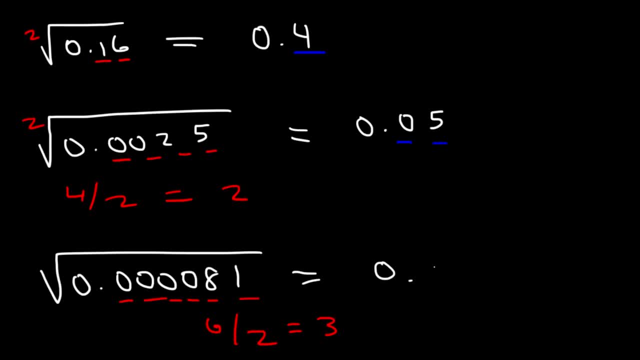 the square root of 81 is 9, so this is going to be .009. now let's talk about cube roots. what is the cube root of 8? what number times itself? three times 8, 2 times 2 times 2 is 8, which is basically 2 to the third. so therefore, the cube root of 8 is: 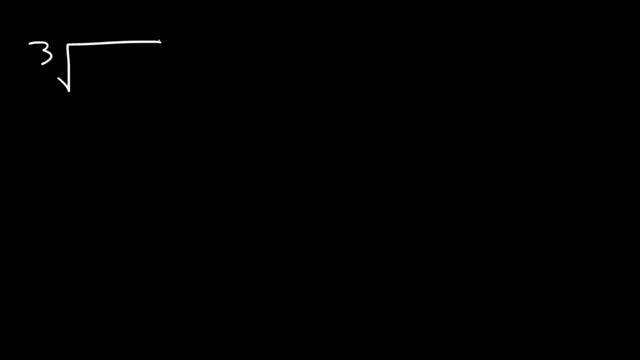 2. now what is the cube root of negative 27? this, it turns out it's negative 3. negative 3, multiplied to itself three times is negative 27. and how about the cube root of 64, but of a negative on the outside? the cube root: 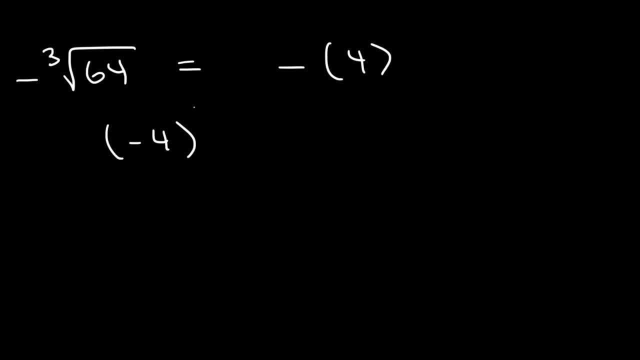 of 64 is for negative 4. x itself three times is negative 64. now what is the cube root of 125 over 216? the cube root of 125 is 5 because 5 to the third is 125 and the cube root of 216 and 6 because 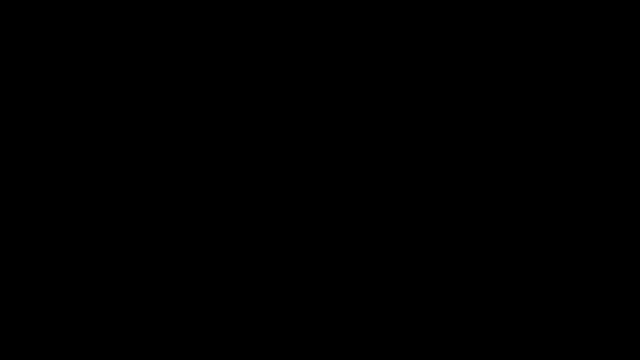 If you multiply 6 three times, you're going to get 216.. Now what is the cube root of a decimal? Let's say 0.008.. Notice that we have three digits to the right of the decimal point. Take that number and divide it by the index number. 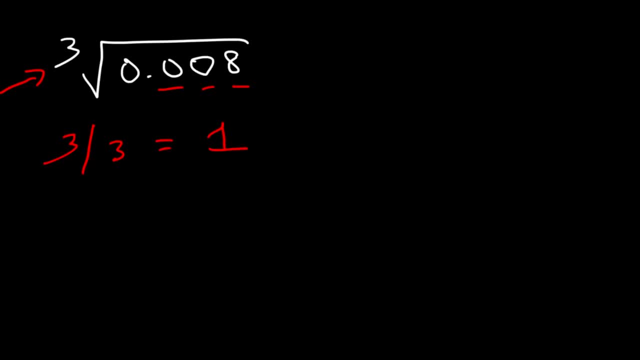 Your final answer should have one digit to the right of the decimal point. Now we know that the cube root of 8 is 2, so this is just going to be 0.2.. As you can see, it has one digit to the right of the decimal point. 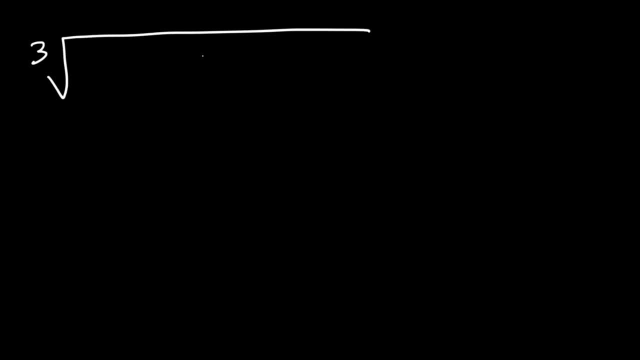 Now, what is the cube root of 0.00027?? Notice that it has six digits to the right of the decimal point. Six divided by the index number 3, is 2.. So our final answer should have a total of two digits to the right of the decimal point.